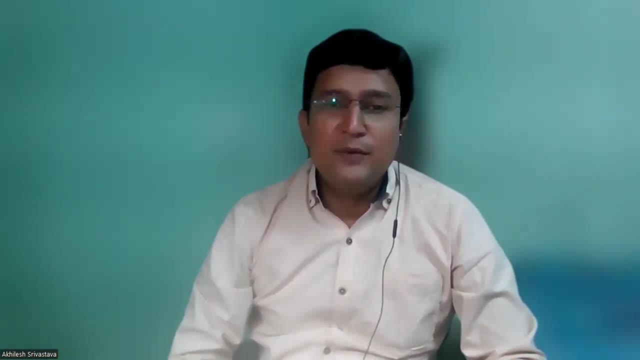 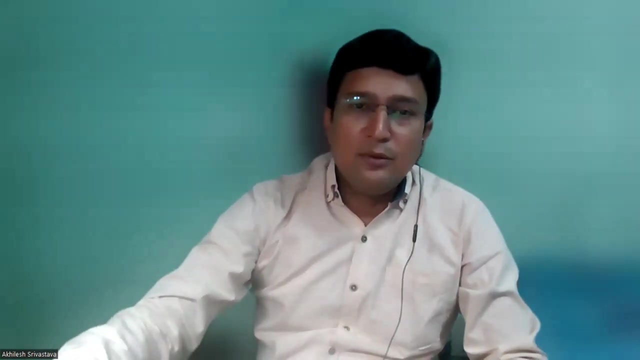 method. It is based on the dynamic programming method, wherein we make every vertex as a mediator one time and find out if we have any shorter length path than the direct path. So let us look at a scenario and find out how to represent a graph in the memory. 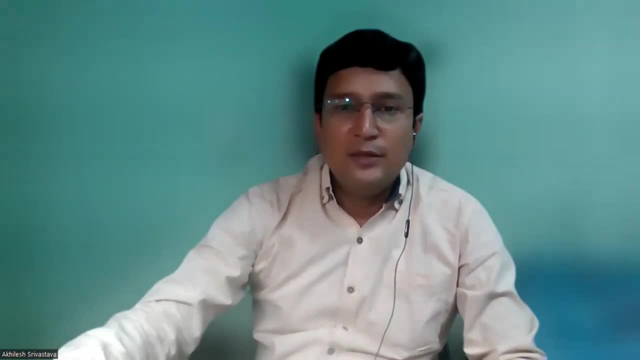 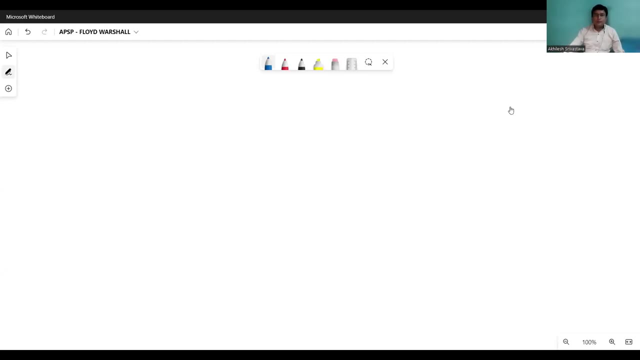 How to use the Warshall algorithm to find the shortest path. Suppose we have a graph and the graph looks like this: Vortex number 1, Vortex number 0, Vortex number 2 and Vortex number 3.. So in this graph we have assigned the weights. 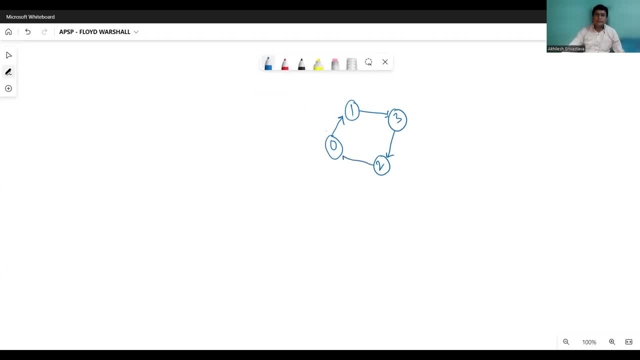 to each of the edge of the graph. Let us say the weights of the edges are: from 0 to 1, we have, let us say, 50,. from 1 to 3, let us say we have 20,. from 0 to 2, let us say we have 10. and then from 2 to 0, let us say: 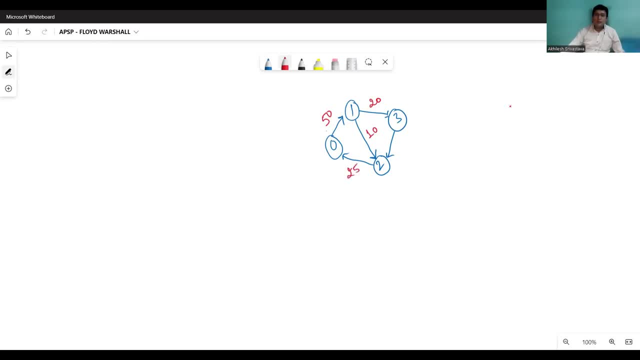 we have 25, from 3 to 2. let us say we have 5 weight. So this is the graph. You can represent this graph by the weight matrix. The weight matrices are similar to that of the adjacency matrix, wherein the connections were represented by 1 and non-connections were represented. 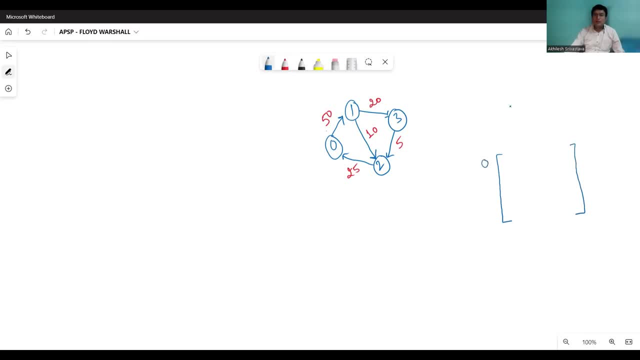 by 0.. So if I have this graph, then if the vertices are 0, 1,, 2, 3,, 0, 1,, 2, 3,, if there is a connection between a pair of the vertex, we will represent that by the weight of that. 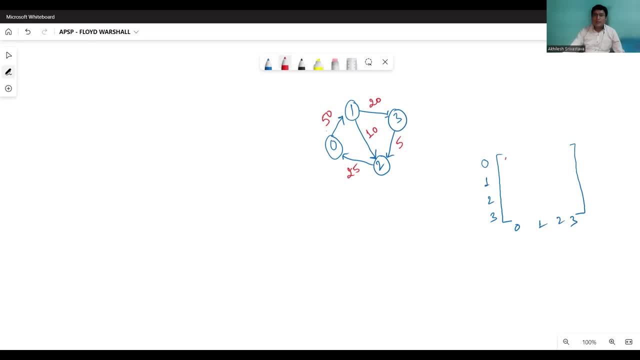 connection. For example, from 0 to 1, we have an edge and it has a coordinate, So we can cost 50. but from 0 to 2, 0 to 3 and 0 to 0 to 1, sorry, 0 to 1, 0 to 2, 0 to 3, we don't have any edge. 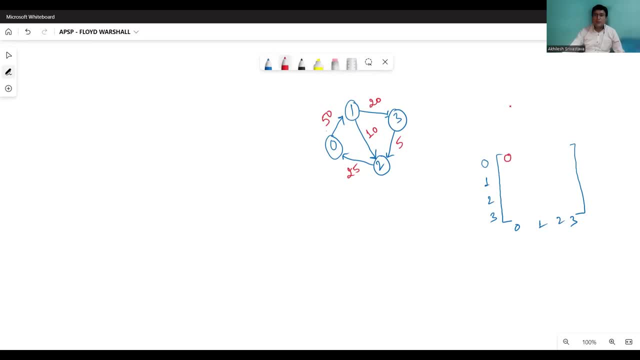 so i'm writing this once again. so 0 to 0: there is no edge, 0 to 1: there is an edge of cost 50. 0 to 2: there is no edge. and 0 to 3: there is no edge. similarly, from 1 to 0: there is no edge. 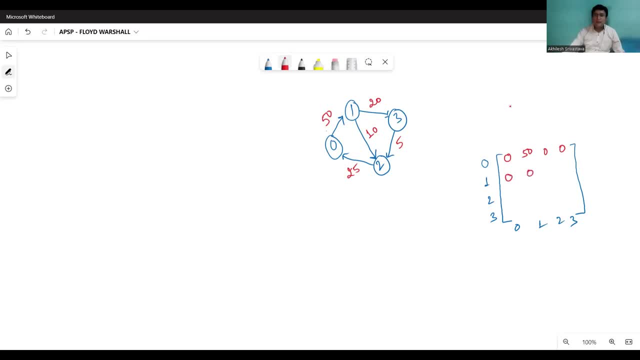 from 1 to 1 there is no edge, but from 1 to 2 we have an edge of cost 10, and 1 to 3 we have a cost edge of cost 20.. similarly, from 2 to 0 we have an edge of cost 25, but there is no other edge from 2. 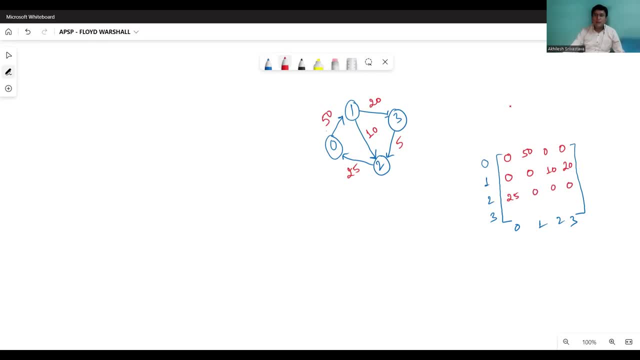 similarly, from 3 to 1, we have 3 to 2. there is a edge, of cost 5 and in all of this scenario, or all other vertices, there is no edge. so this is the weight matrix of the given graph and if you have to find out the- uh all pair- shortest path, it means we have to find out the shortest part. 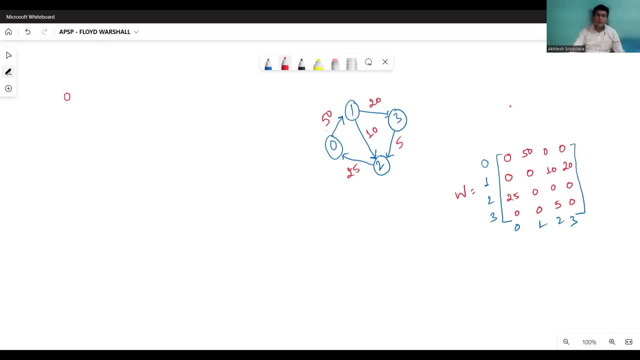 between every pair of the vertex, that is, we have to find out the shortest path between 0 to 1, 0 to 2, 0 to 3. then we have to find out the shortest path between 1 to 0, 1 to 2, 1 to 3 and from 2 to 0, 2 to 1 and 2 to 3 and 3 to 0, 3 to 1 and 3 to 2. 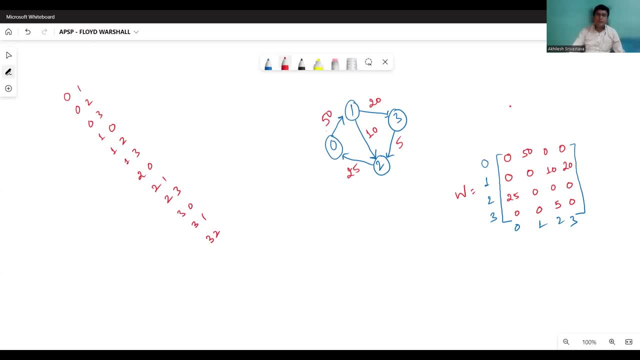 so these are all possible pairs between which we have to find out the shortest path for finding out. warschall has suggested a method that you first prepare the distance matrix. and the distance matrix can be prepared like this: if i have all the weights positive and there is no negative weight. 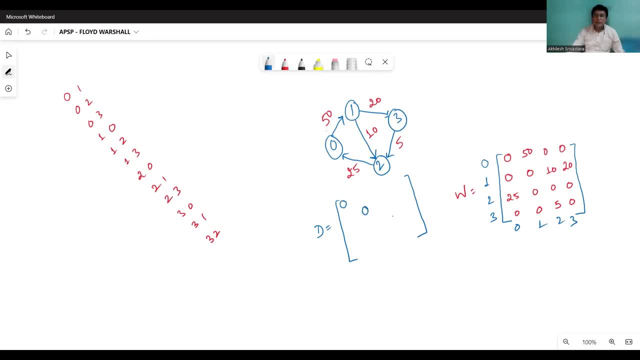 then i can keep all the diagonal elements as zero, meaning that if i have the vertex from one to one or we have the entry from one to one in the distance matrix, obviously you can read in zero time, since we have kept the distance of all the diagonal entries as zero, so diagonal. 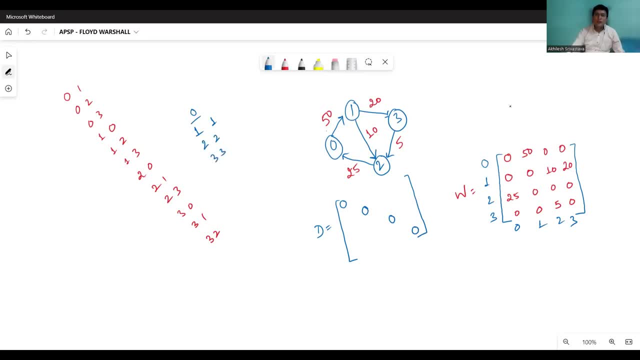 entries will be representing one: one, two, two, three, three, and the first one will be representing the zero- zero. so let's mark the vertex number so that it becomes easier for us to make the entries. and then for all the positive entries are kept as same. for example, we are keeping: 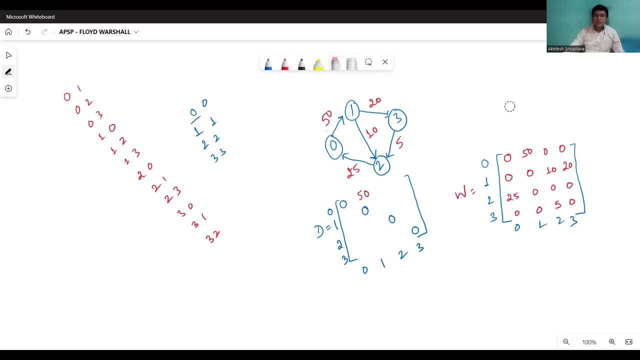 all the positive entries greater than zero entries at the place, wherever they are, and then we are making all other entries in the table as infinite. it means, if i have the zero entry in the weight matrix for the distance matrix, it looks like that we we are not able to reach from the source vertex to the destination vertex, for example. 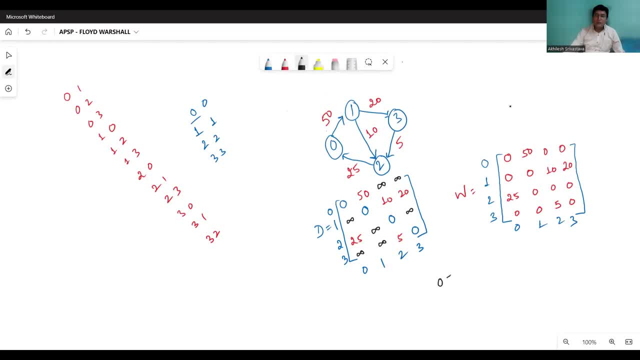 here in this matrix, i can say that i cannot reach from zero to three. i cannot reach from zero to three. similarly, i cannot reach from one to zero. i cannot reach from two to one and two to three. i cannot reach from three to one. so three to zero and three to one. because these entries are 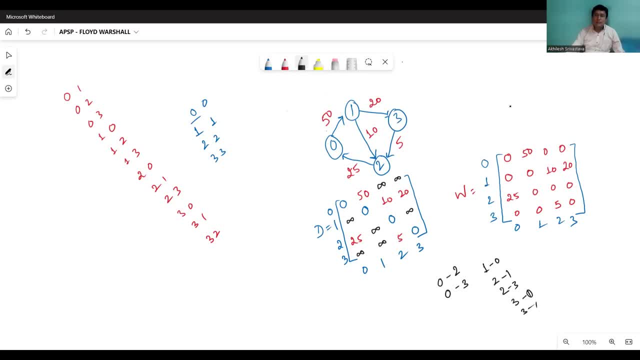 infinite. so making the entries infinite initially means that initially these vertices are not approachable. it means the vertices have no connections as of now. but the varchel has suggested that you should take every vertex once as a mediator and find out if the path exists via that vertex, for example. 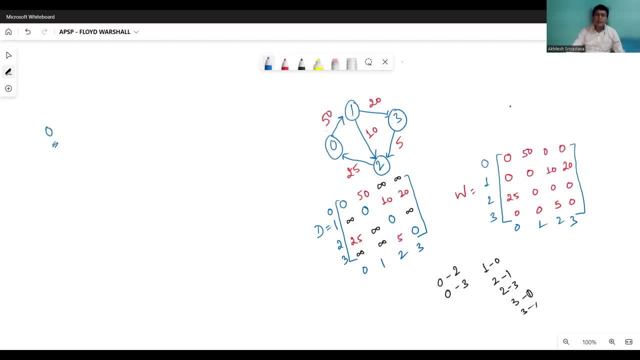 if i select the vertex number zero as a mediator, then you can see that if i have the vertex zero as a mediator, so two to one entry, which is initially, initially infinite. this is, you can see that this is infinite, but i, if i take the vertex number zero as a mediator, 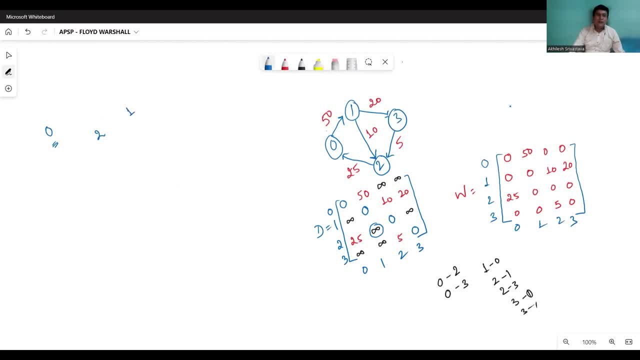 then i can reach from two to one via zero, because there is a path from two to zero and there is a path from zero to one. so two to zero path has a cost 25 and zero to one has a cost 50.. now if i have- uh, if i take another example of for this varchel algorithm, let's take another. 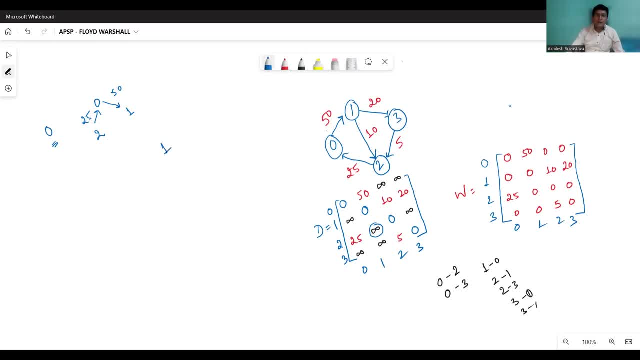 vertex as a mediator. let's say we are taking vertex number one as a mediator, so i cannot reach from zero to two directly. but i have a method of reaching from zero to two via one. so zero to two can be reached via one, as you go first from zero to one, which has a cost 50, and then you go. 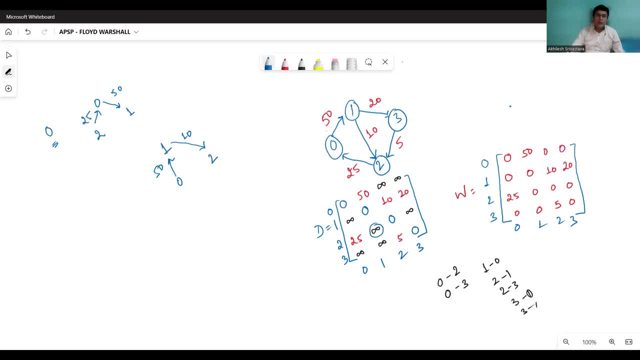 from one to two, which has a cost 10.. so all together you can reach from zero to two in 60 amount of the distance. so you should update your matrix accordingly. so either the path is, either the direct path is minimum. so if i have a dij entry in the matrix, 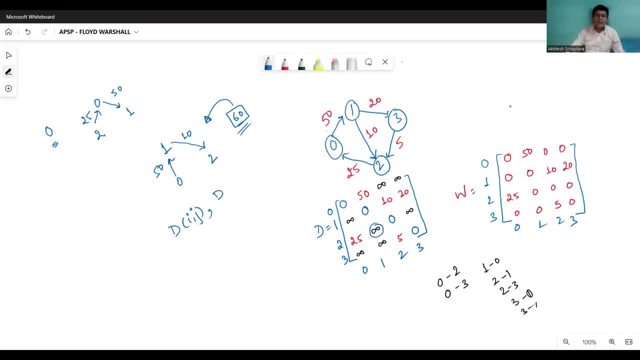 so either that is minimum or if i take a vertex k as a mediator, then you go from i to k and then you go from k to j and you add the cost of these two or you add the distance of these two edges and maybe that this is minimum. so either this will be minimum or this one. if i take a scenario, 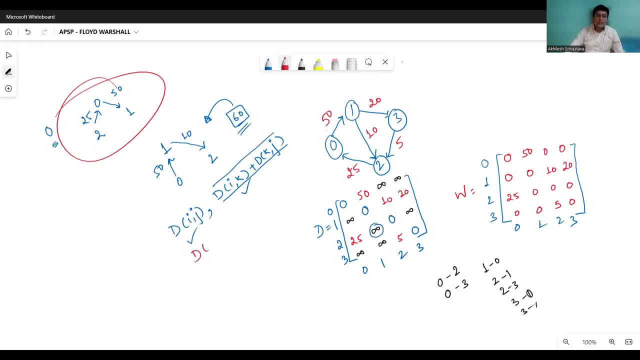 of this one. what we took, the i- j was like two, zero and we took two one. sorry, i was two and j was one and the k was zero, the vertex that has been taken as a mediator is zero. so if i take the zero number vertex as a mediator, so if i first go from two to zero and then i go from zero to one, 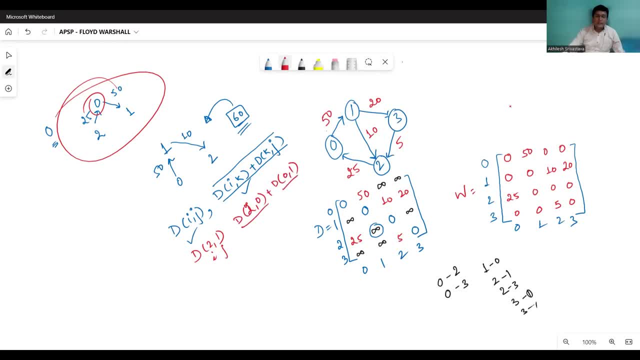 and then we add up these two costs. so either the distance between two to one, which is infinite in the table or in the matrix, or two to zero, has a cost 25 and this has a cost 50. so if i add these two means, 25 and 50, it becomes 75, which is the smaller one as compared to the infinite. 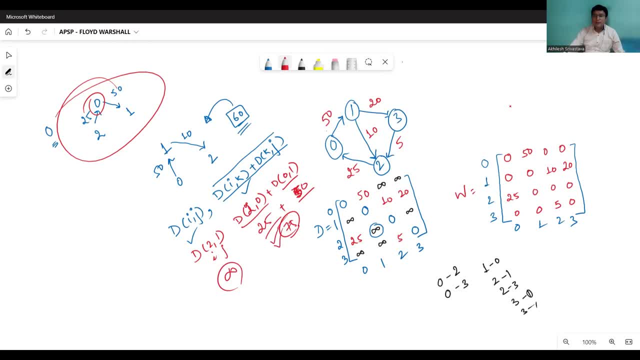 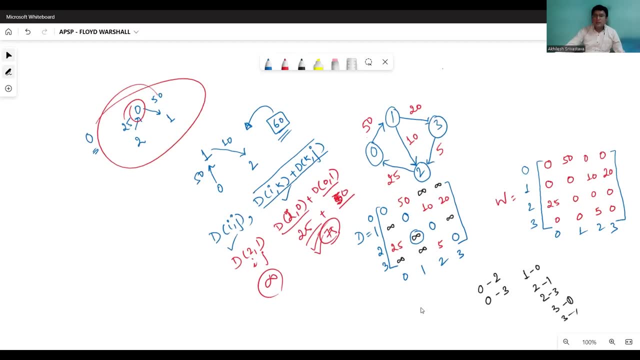 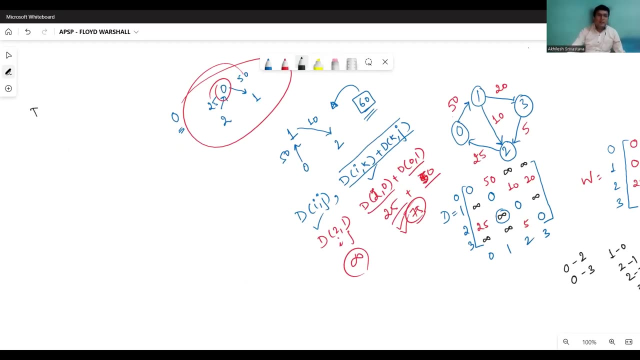 so i will take or i will update the matrix entry as 75, so at a time you will take one vertex as a mediator and you will keep going like that. you have to take every vertex as a mediator at some point of time. so let's say we have the distance matrix available. we have already formed 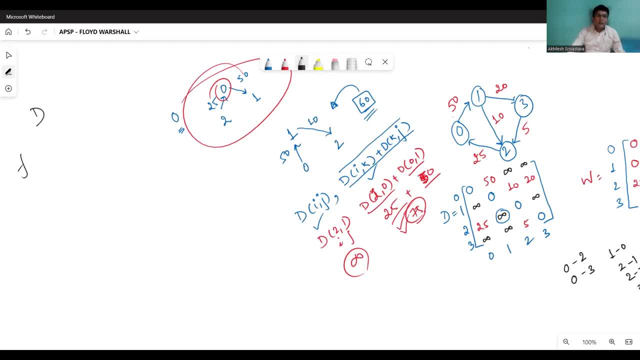 the distance matrix, let's say, then we will have to take every vertex as a mediator. so let's write the algorithm. let's say that we have a k which is a mediator, so for k equals to 0 to n minus 1, 2, let's say n is representing the number of the vertices and the number of. 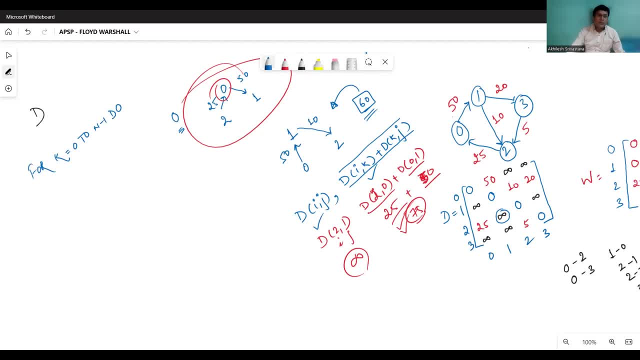 the vertex is ranging from 0 to n minus 1. so if you take k as 0, you will have to see all the entries of the table. so that's why our nested loop will be working here. so for i equals to 0- 2. 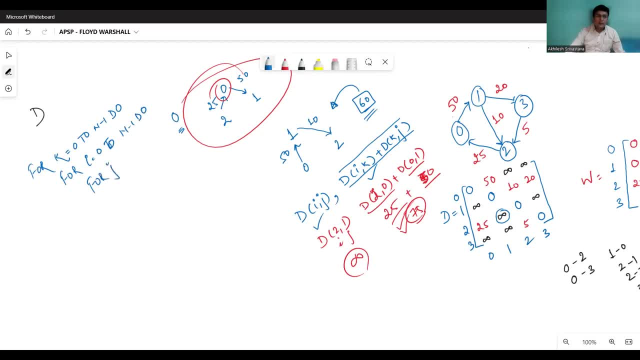 n minus 1- 2 and for i, for j is equal to 0 to n minus 1, 2. so let's say the i is representing the row number and the j is representing the column number. you will apply a formula if you have to see the dij entry. so either the dij is directly minimum or dik plus dkj entry is: 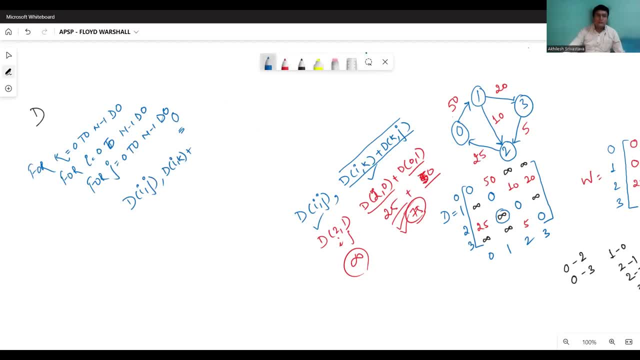 so let me erase this so that we have a sufficient space to write. so either this is minimum or that is so whichever is. whichever of these two is minimum, that will be updated as dij. the matrix entry from d to ij, d in d from i to j will be updated with this form. 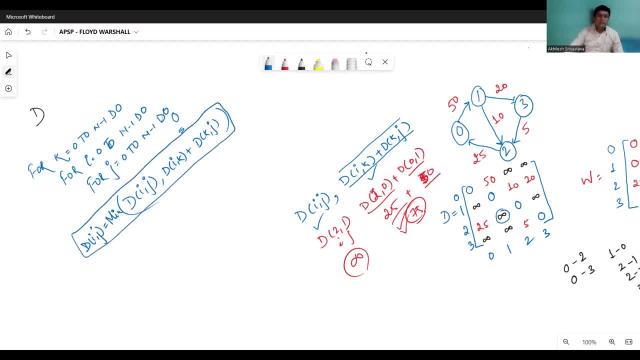 so this line will be inside the inside the line. so we please bear with me because i have the indentation has gone wrong this way because it is written externally before us, so offweb reference problem. so in order to useless matrix entry. so if you have selected k is equal to 0, you will look for all the entries in the table. 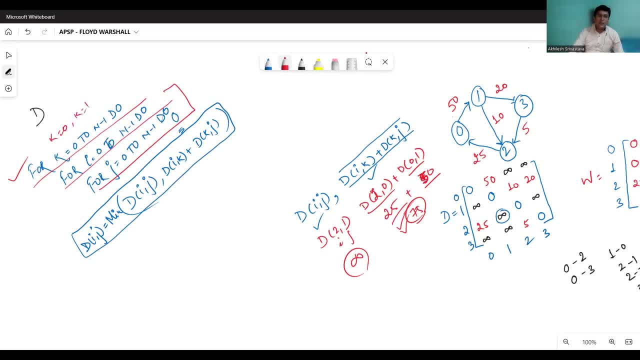 or in in the matrix and then you have k equal to one, then again you will look at all the entries in the matrix. if you have k equals to 2, you will transfer all the entries to number 3. so if you have k equals to 2, this matrix, entry of the matrix we took, and in that another turn we have to expand the. loop as we are taking. these two are the matrix entries out. it will be onừ parametrically. i mean put the case moderately in each series matrix, as we have, k equals to 2.5, because we are know which one toeling in here. 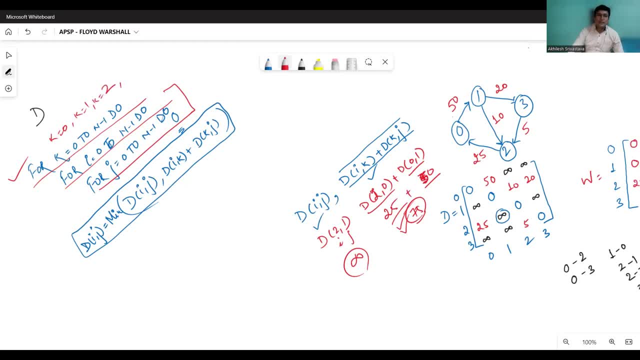 and then showing you that, because that is the answer we want to solve to the question now. so let's see the numbers right now. this is three times J and then say now, if you have all the entries, three, If you have k equals to 2, you will once again see all the matrix entries. 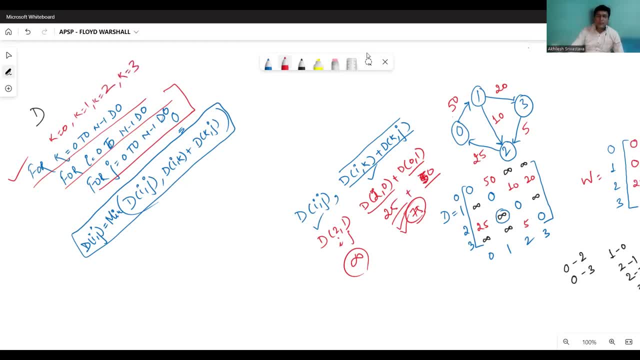 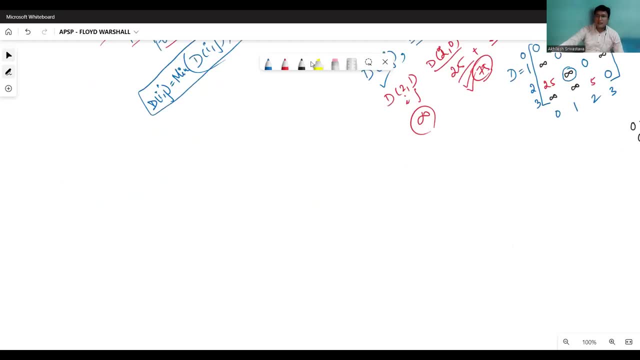 And if you have k equals to 3, you will see all the matrix entries. So this is one part of the algorithm, But when you will implement this you will find some of the difficulty. So let me explain those difficulties also a priori, before going to code this. 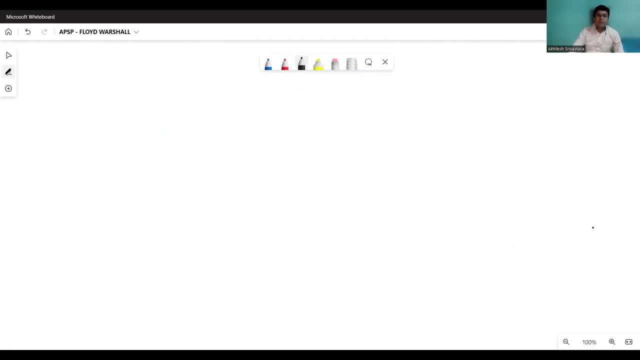 So let's say you have a weight matrix and you have to convert this weight matrix to the distance matrix, If I take the same example that we took here. Fine, so we have a weight matrix and you have to convert this weight matrix to the distance matrix. 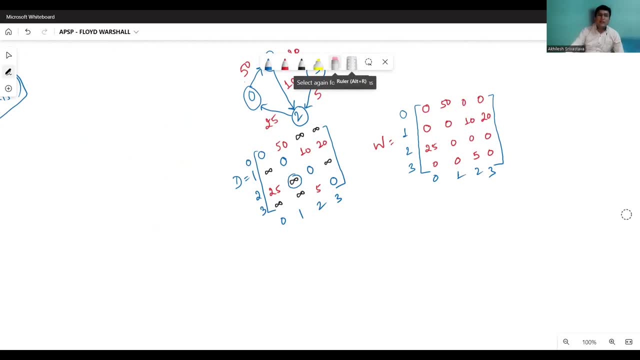 So, while conversion of the weight matrix to the distance matrix, whenever you are taking the entries in the weight matrix, at the same time you can set the distance matrix also. Now you will have to convert some of the entries as infinite. Fine, so I'm just underlining that these are the entries which will be set as infinite in the distance matrix. 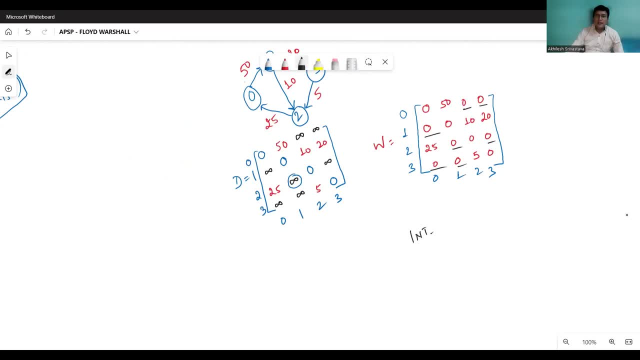 So how to set the infinite? One of the method is that you select the integer maximum, if you are representing the integer maximum as the maximum limit of the integer. So this is one of the way you can set the infinite, But there is a logic of getting the maximum limit of the integer. 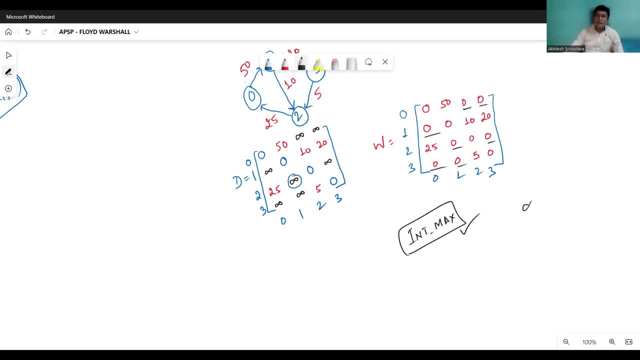 So you can set the infinite as the maximum limit of the integer if you are representing the integer maximum as the maximum limit of the integer. So if you are getting this as a failure at some point of time, for example, if you have one of the entries infinite and you are adding another entry as the infinite, 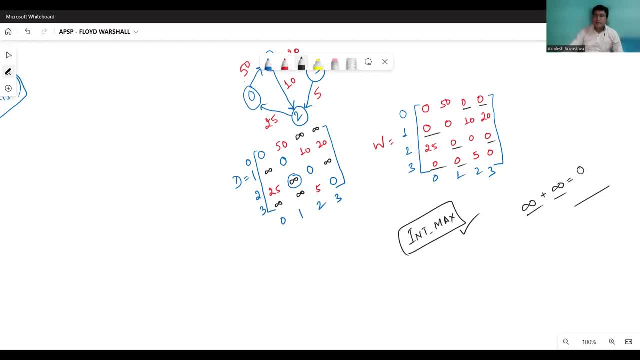 So these infinite plus infinite, if these are integer max and integer max in the implementation, when you add these two values, these will become zero, because you know that if you cross the limit of the integer, a cyclic process is followed and you go towards the negative side. 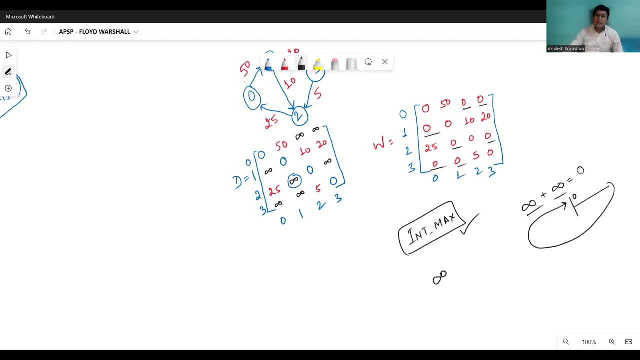 So if you add the same number of same value And any other value- let's say you are adding 52, the infinite- then you will end up with the negative. So neither do you require this negative value nor you want this zero to appear. 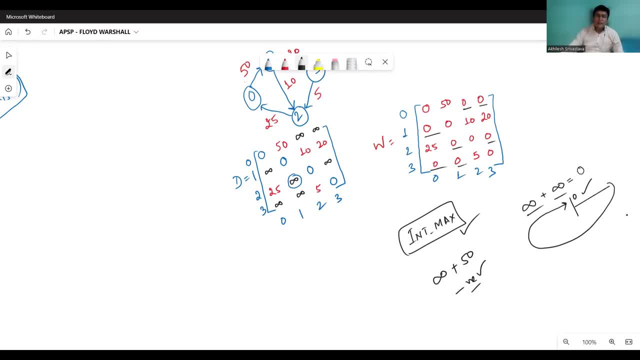 So this will be an error actually, And the computations will find some of the errors in the computer. So what should you do? that You should take the, the infinite as integer max divided by two, because if you add the integer max divided by two with 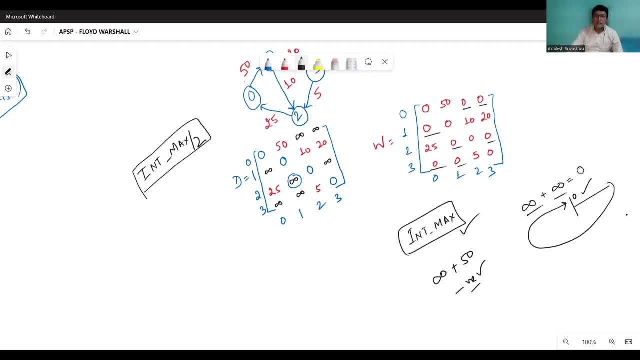 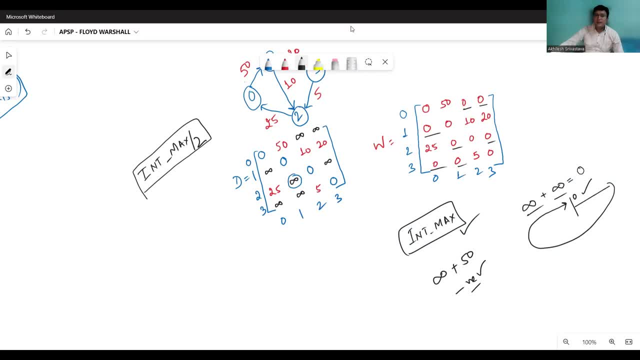 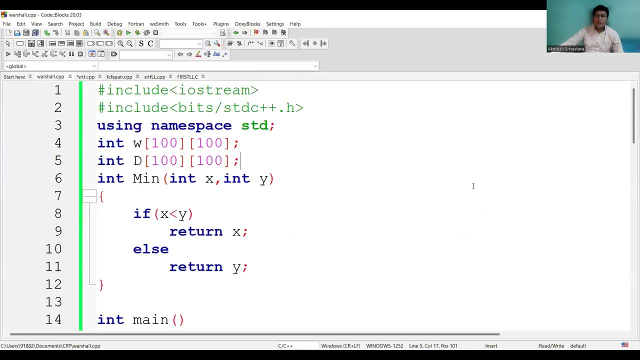 we can implement this algorithm very well. now let's look at the code for this. so here is the code, and in this i have taken the two, two matrices: the big size matrix of w and the d. w is representing the weight matrix and d is representing the distance matrix. 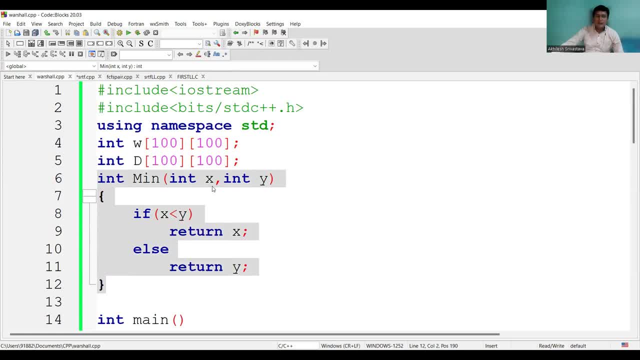 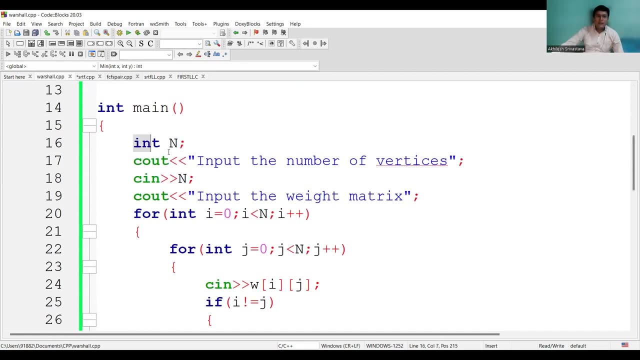 since you require the minimum. so i have just written a small function of the minimum which has two parameters in it: x and y. if x is less than y, it will return x, otherwise it will return y. now, coming to the main, where i have, where i have taken the input of the number of: 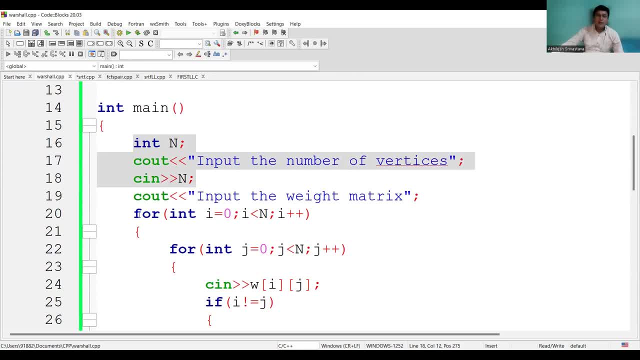 vertices by the user in n variable. after this i am getting an input of the number of vertices by the user in n variable. after this, i am getting an input of the number of vertices. weight matrix. so the weight matrix can be taken as a number with the help of the two two nested: 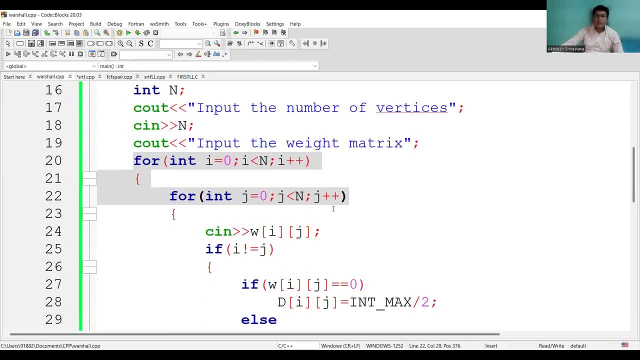 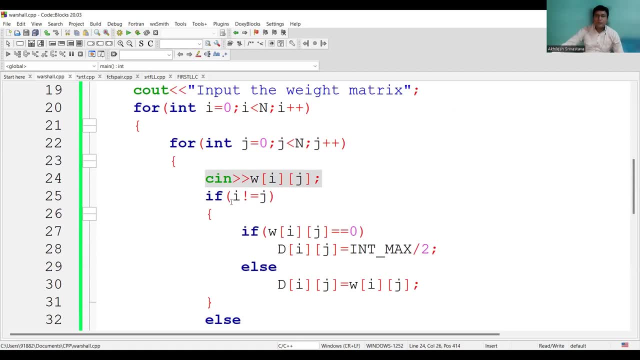 loops i and j. nested loop. i is representing the row number and j is representing the column number. the weight matrix has been input in w now if we are converting this weight matrix to the distance matrix at this point of time. so if i is not equal to j, it means that it is not a diagonal entry. so 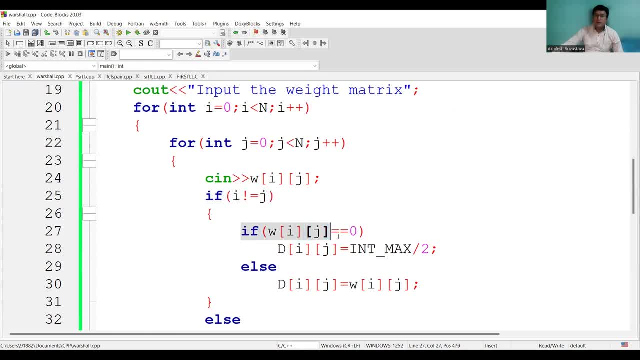 if i is not equal to j, it means that it is not a diagonal entry. so if i is not equal to j, it means that it is not a diagonal entry. if this is not the diagonal entry, if this is not the diagonal entry, you have to do two things. if the weight matrix is representing 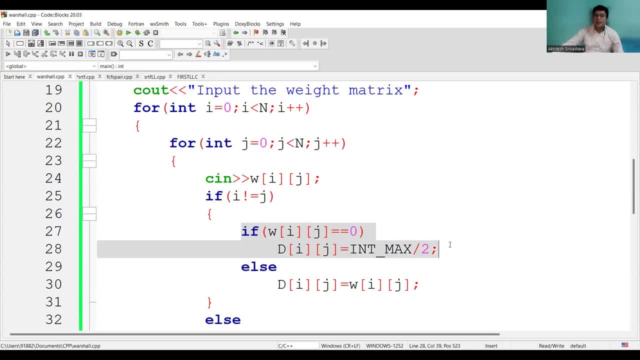 you have to do two things. if the weight matrix is representing, you have to do two things. if the weight matrix is representing zero, it means you have to zero. it means you have to zero, it means you have to set that value as the infinite. so integer max. 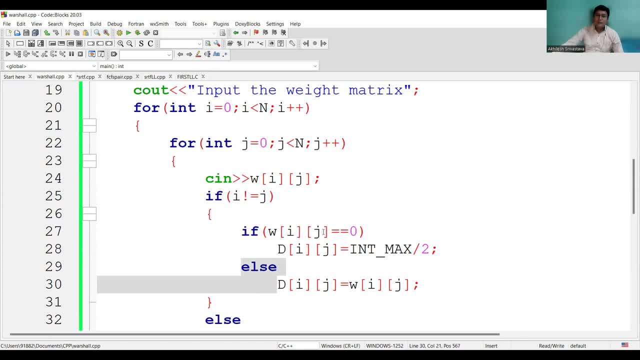 set that value as the infinite, so integer max set that value as the infinite, so integer max divided by 2 is giving you the infinite. divided by 2 is giving you the infinite. divided by 2 is giving you the infinite and if it is not, zero value. 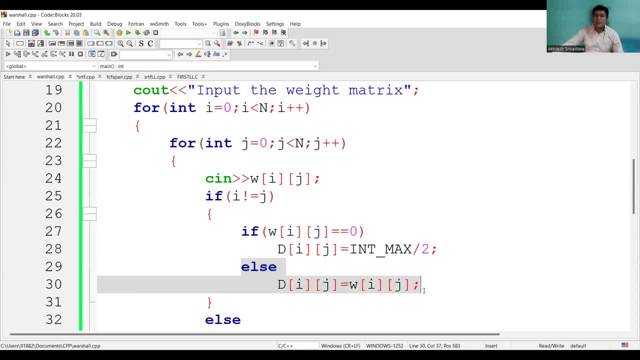 and if it is not zero value? and if it is not zero value, then you will keep that value unchanged. so then you will keep that value unchanged. so then you will keep that value unchanged. so, whatever is the value in the wij, whatever is the value in the wij. 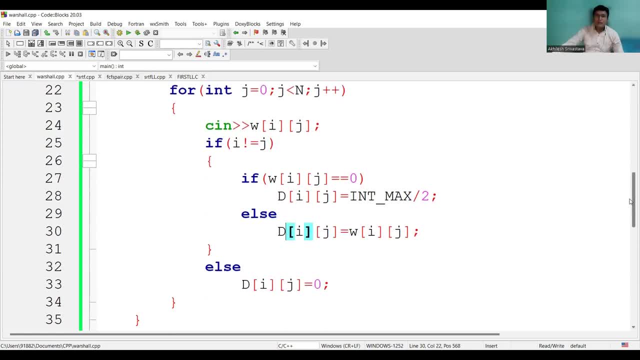 whatever is the value in the wij, the same will be there in the distance, the same will be there in the distance, the same will be there in the distance. matrix as well, matrix as well, matrix as well. but if we have the diagonal entry, then. but if we have the diagonal entry, then. 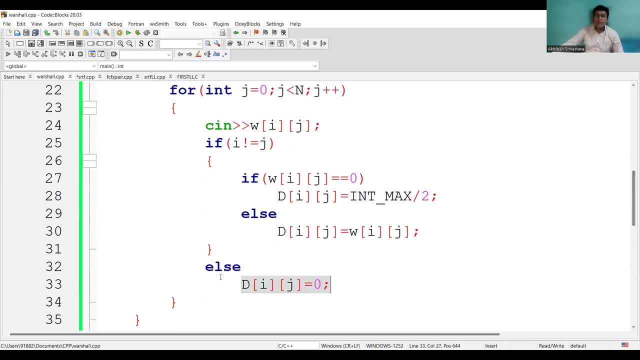 but if we have the diagonal entry, then that diagonal entry will be set as that diagonal entry will be set as that diagonal entry will be set as zero. or you can say that if, even if you zero, or you can say that if, even if you zero, or you can say that if, even if you leave it as such, because in the weight 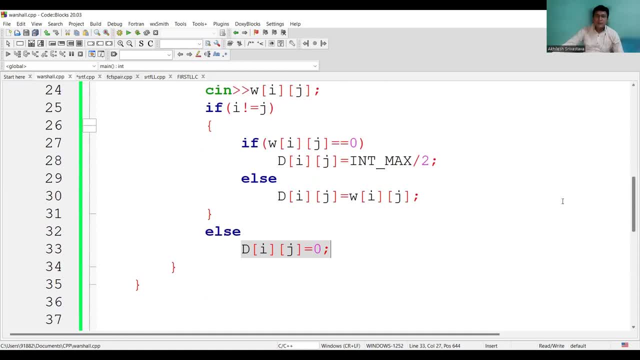 leave it as such. because in the weight, leave it as such, because in the weight matrix also, this value will be matrix also this value will be matrix also this value will be zero. so you are setting that zero, so you are setting that zero, so you are setting that b i j entry has been set as zero. 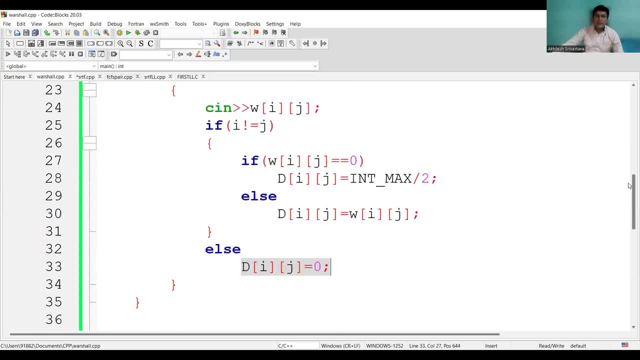 b i j entry has been set as zero. b i j entry has been set as zero for the diagonal. so we have formed the for the diagonal, so we have formed the for the diagonal, so we have formed the distance matrix, and then distance matrix, and then distance matrix, and then comes the uh varshel algorithm, the actual. 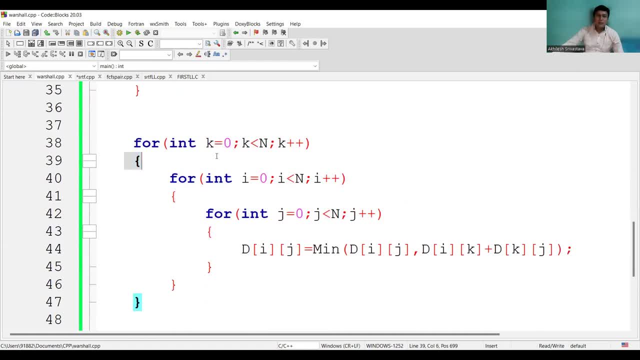 comes the uh varshel algorithm. the actual comes the uh varshel algorithm. the actual varshel algorithm. varshel algorithm, varshel algorithm. but in three loops are taken: the, but in three loops are taken. the but in three loops are taken. the outermost loop is telling that 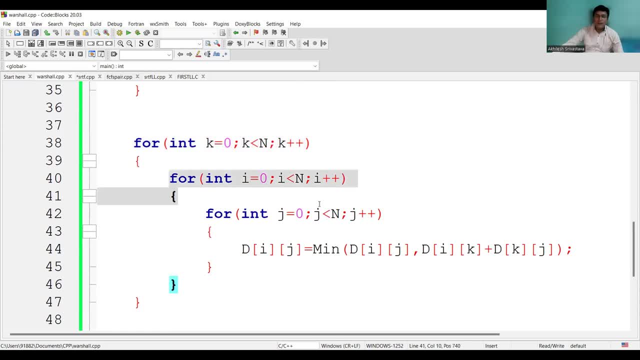 outermost loop is telling that outermost loop is telling that we are taking one vertex as a mediator. we are taking one vertex as a mediator. we are taking one vertex as a mediator at one point in time, at one point in time, at one point in time. and then this: these two nested loops are: 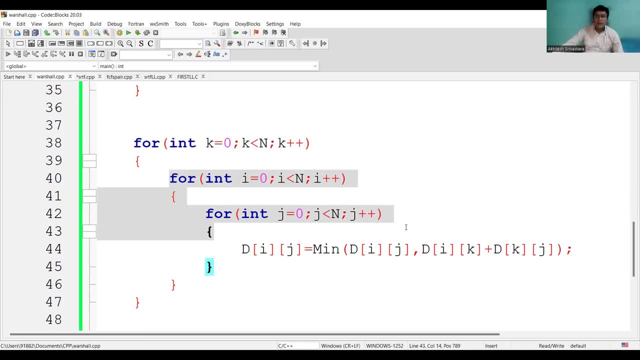 and then this: these two nested loops are, and then this: these two nested loops are saying that we will look for all the saying, that we will look for all the saying, that we will look for all the entries in the entries, in the entries in the weight in in the distance matrix for 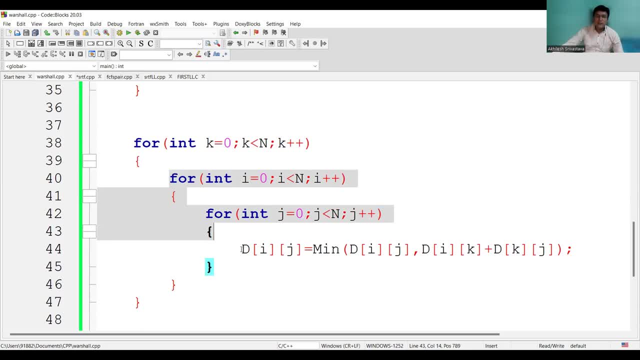 weight in in the distance matrix for weight in in the distance matrix for every selected, every selected, every selected mediator, vertex, mediator, vertex, mediator, vertex. the formula says that you have either the. the formula says that you have either the. the formula says that you have either: the dij is minimum directly. 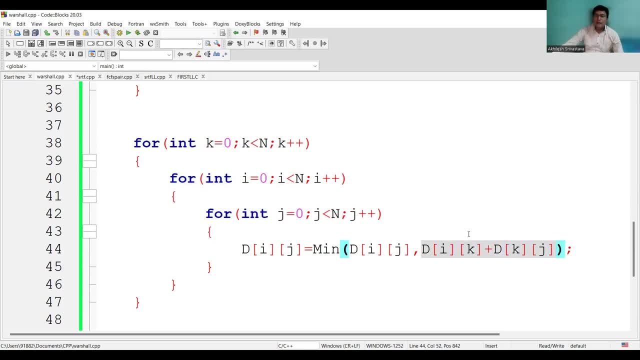 dij is minimum directly. dij is minimum directly. or you go through k and the path for, or you go through k and the path for, or you go through k and the path for. from i to k and k to j added together. from i to k and k to j added together. 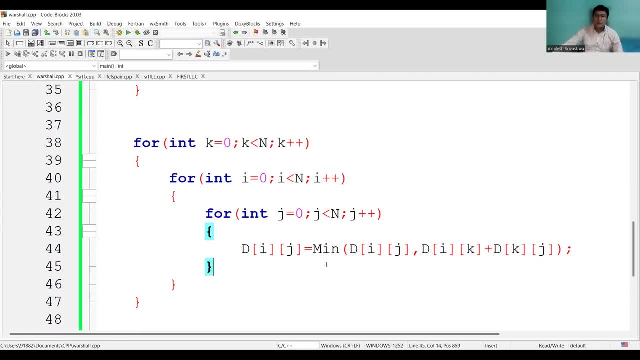 from i to k and k to j added together is is is. so you're finding out the minimum of these. so you're finding out the minimum of these. so you're finding out the minimum of these. two and whatever is the value is set. two and whatever is the value is set. 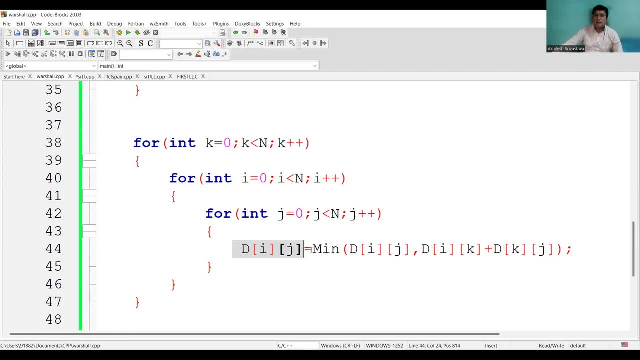 two and whatever is the value, is set at that d. or you have updated the at that d, or you have updated the at that d, or you have updated the distance matrix through this formula. finally, you will print this matrix. finally, you will print this matrix. finally, you will print this matrix, the dij matrix. 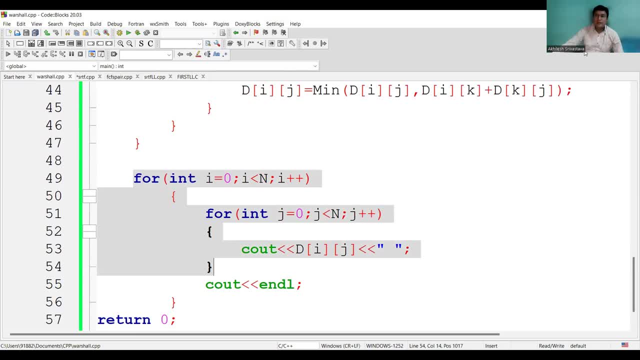 the dij matrix. the dij matrix. let's look at this algorithm. let's let's look at this algorithm. let's let's look at this algorithm. let's run this algorithm and see if this run this algorithm. and see if this run this algorithm and see if this works correctly. 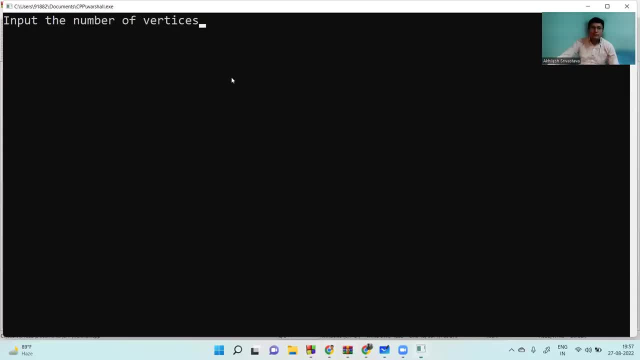 so i'm running this. so i'm running this. so it's asking to enter the number of the. so it's asking to enter the number of the. so it's asking to enter the number of the vertices, vertices, vertices. uh, let's go to. uh, let's go to. 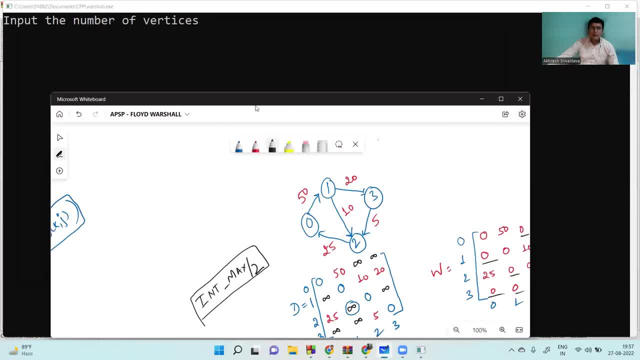 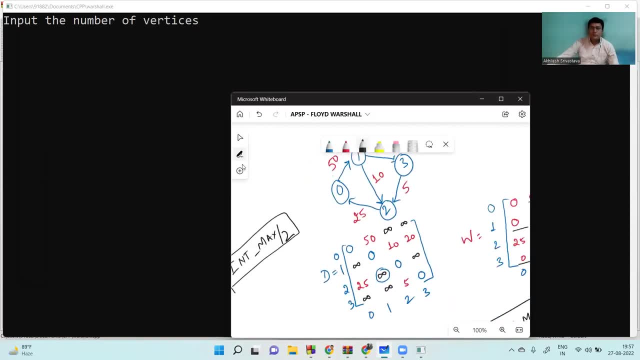 uh, let's go to the whiteboard, where we have taken the whiteboard, where we have taken the whiteboard, where we have taken an example, and with the same example, an example and with the same example, an example and with the same example, i will take the inputs. 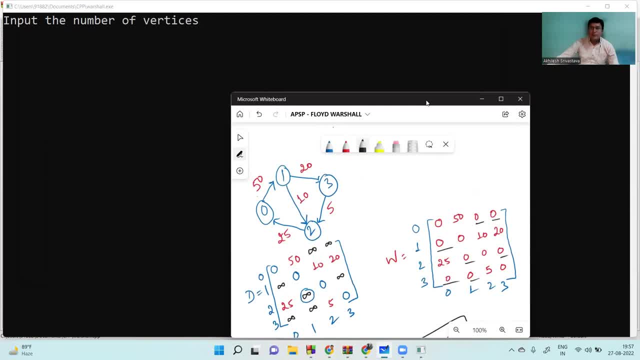 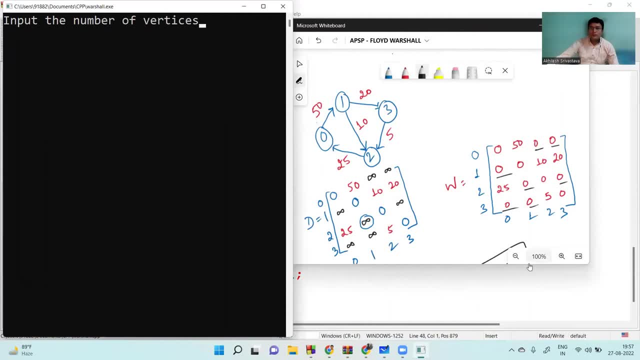 so we have a weight matrix for the graph. so we have a weight matrix for the graph. so we have a weight matrix for the graph. given, given, given, we'll input the same weight matrix. so this is the output and this is the. so this is the output and this is the. 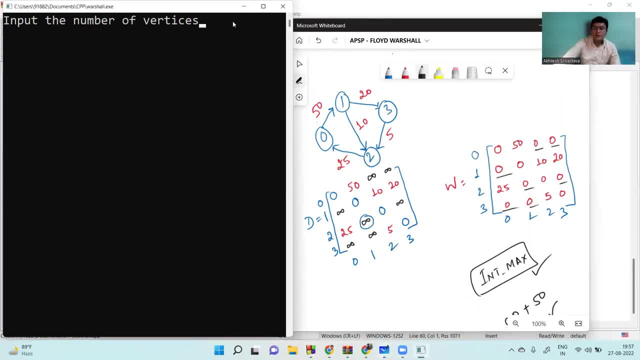 so this is the output and this is the graph: graph, graph. so it's asking about the number of the. so it's asking about the number of the. so it's asking about the number of the vertices: it is four. number of the vertices: it is four. number of the. 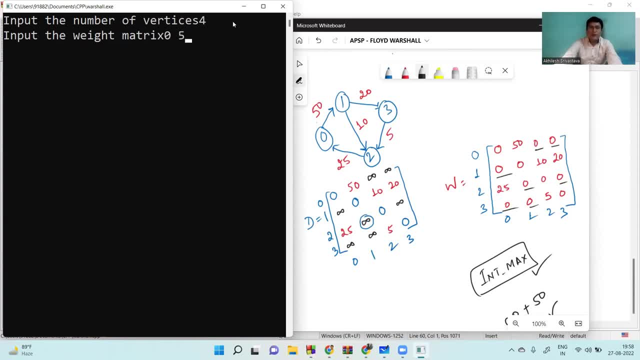 vertices. it is four. number of the vertices here. vertices here. vertices here: the weight matrix is zero. fifteen the weight matrix is zero. fifteen the weight matrix is zero, fifteen. zero and zero, zero and zero, zero and zero. then zero, zero, ten and twenty. then zero, zero, ten and twenty. 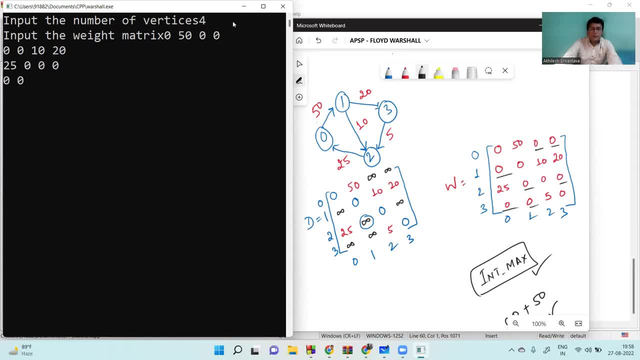 then zero, zero, ten and twenty twenty five, zero, zero, zero, twenty five, zero, zero, zero, zero, zero, twenty five, zero, zero, zero, zero, zero, zero, five and zero five and zero five and zero. so these are the updated entries you can. so these are the updated entries you can. 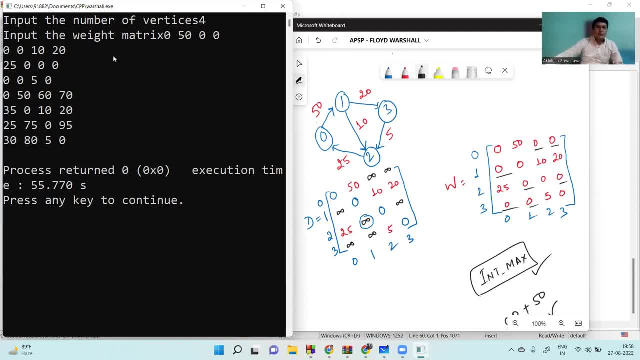 so these are the updated entries. you can see that the input matrix is zero fifty. see that the input matrix is zero fifty. see that the input matrix is zero fifty. zero, zero, zero, zero, zero, zero. but when you got the output the first? but when you got the output the first? 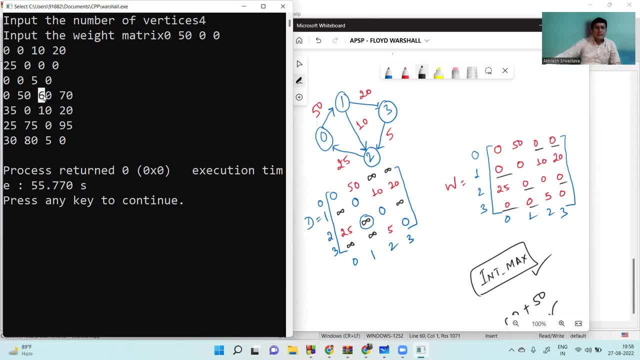 but when you got the output, the first row has two updated values. row has two updated values. row has two updated values. sixty at zero- two position. sixty at zero- two position. sixty at zero- two position and seventy at zero- three position. so, and seventy at zero- three position, so. 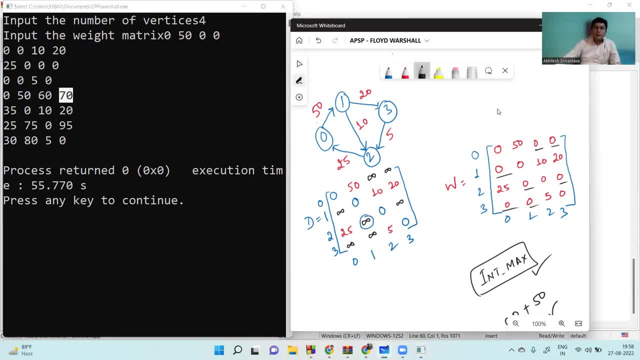 and seventy at zero three position. so let's verify if these entries are. let's verify if these entries are. let's verify if these entries are correct or not correct or not correct or not. so the zero two entry is sixty, so the zero two entry is sixty. 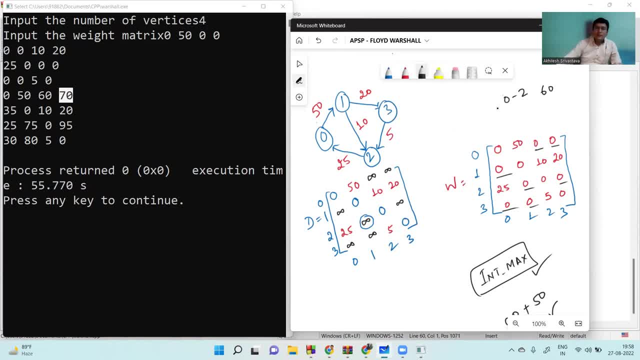 so the zero two entry is sixty. how did we get the zero two entry as? how did we get the zero two entry as? so this has been verified. 0 to 3 entry is 70. so let's verify if it is correct. so if you go via 1 to 3, 0 to 1 and then 1 to 3, this is 50 plus 20, 70. this is also got verified. 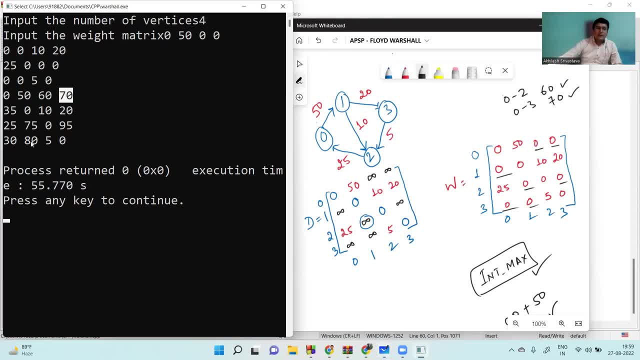 you can take any other random value which has been updated. let's take this value: 3 to 0. okay, so 3 to 0 is one of the entry which has been updated. so 3 to 0 can be reached via 2. yes, so if you go from 3 to 2 and then 2 to 0, the entry is 5 plus 25. that is set. so this is.